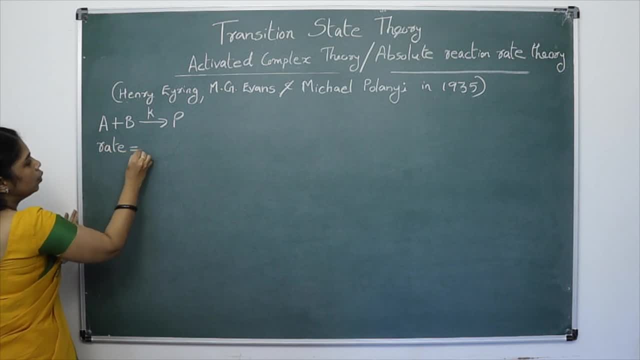 it as k, So 2, now that we write this particular quieren cassiop мощ 이면 A plus B, 곶 rate law, as rate is equal to k, into concentration of A, into concentration of B. But transition state theory says for this bimolecular reaction, the mechanism should: 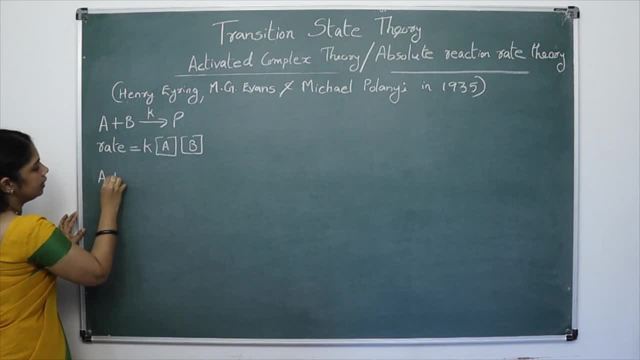 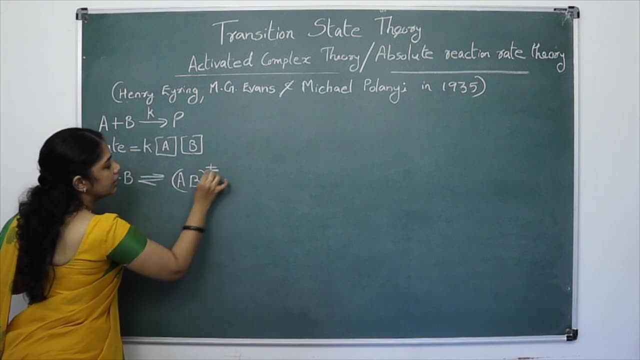 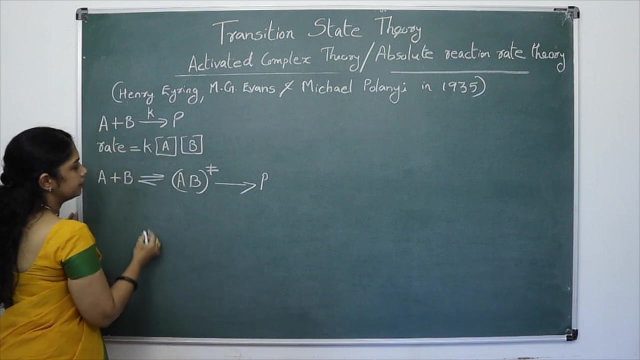 be like this: that is a plus b in equilibrium, with a- b double dagger, which reacts in an unimolecular fashion to give the product. So here capital K double dagger is a equilibrium constant and I denoted k 2 as the. As per the transition state theory, this is a mechanism of a bimolecular reaction. They 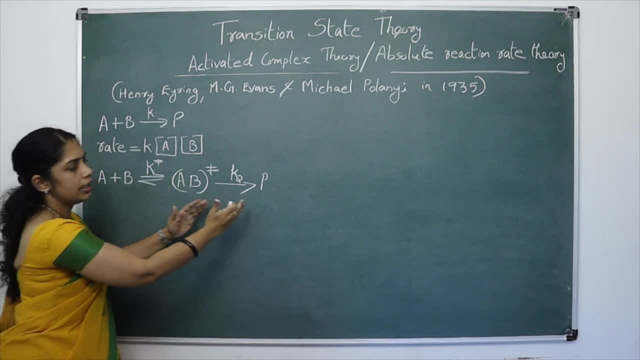 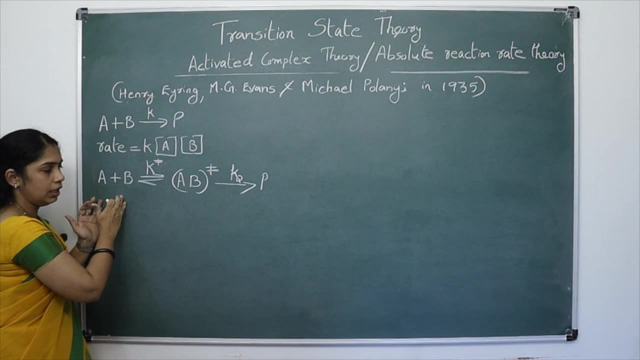 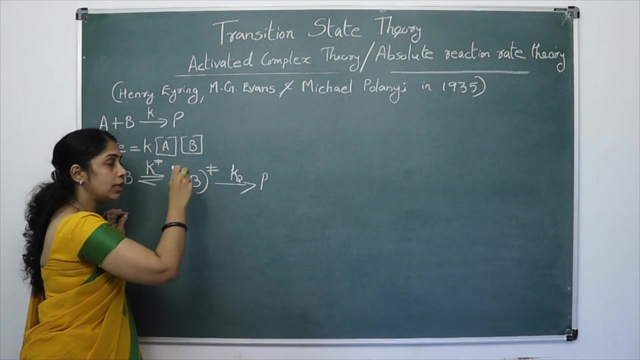 place an activated complex in between the reactants and the products And this activated complex will be in equilibrium with the reactant. And also this activated complex reacts in a unimolecular fashion to give the product. So this is a mechanism as per transition. 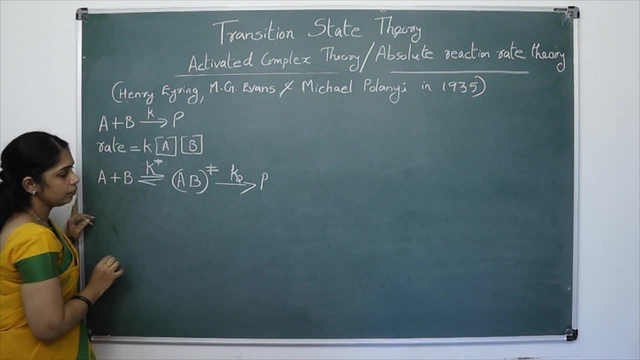 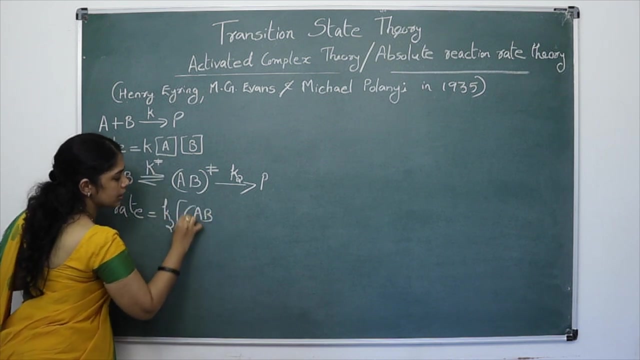 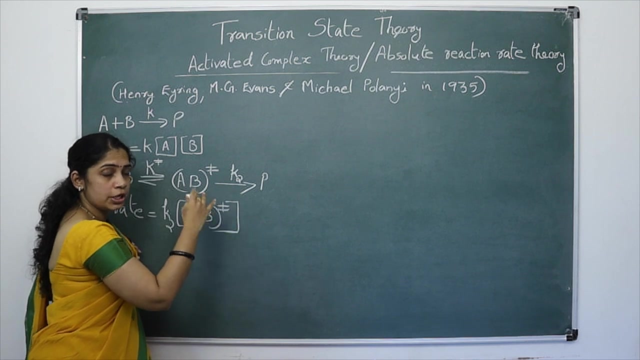 state theory for this reaction. And for this reaction what will be? the rate? Rate is equal to k, mu, k 2 into concentration of activated complex, That is, concentration of a, b double dagger, Because rate always proportional to the concentration of the reactant And rate is here the rate. 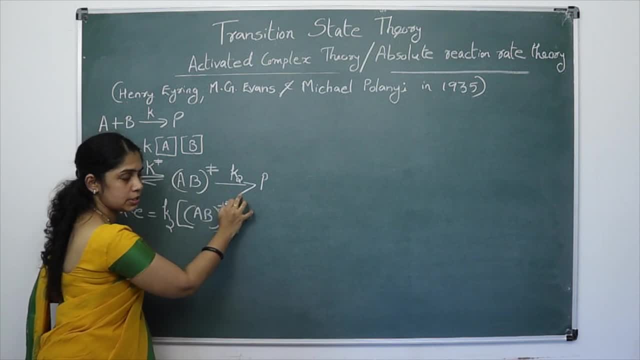 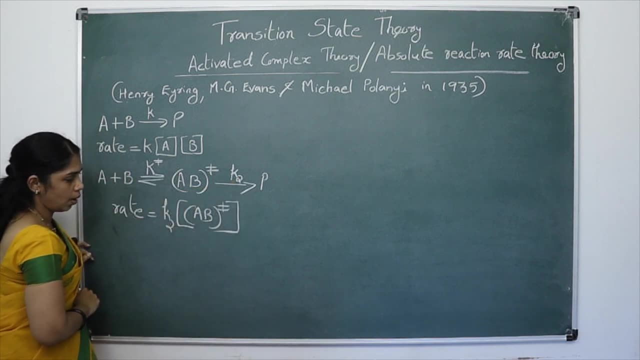 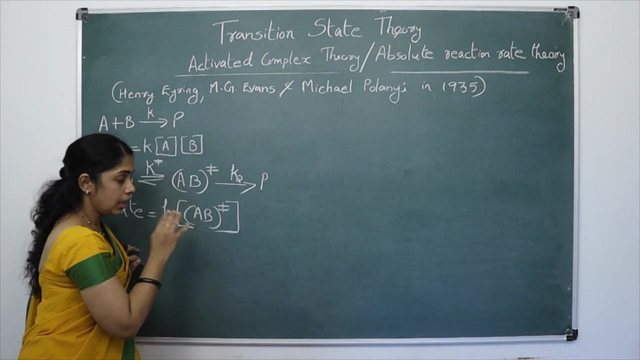 determining step is the. this is the rate determining step. There is formation of the product And rate will be equal to k 2 into concentration of this activated complex. And we know that concentration of activated complex is not a real thing, So we can convert this term. 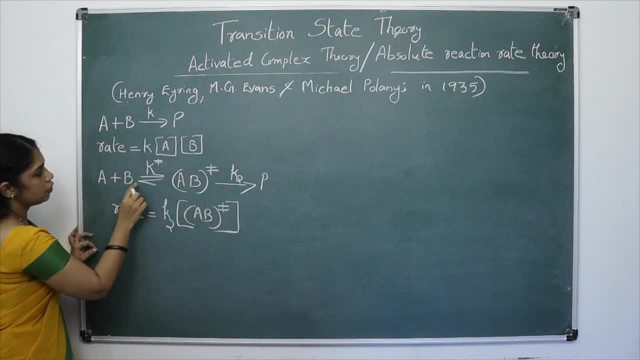 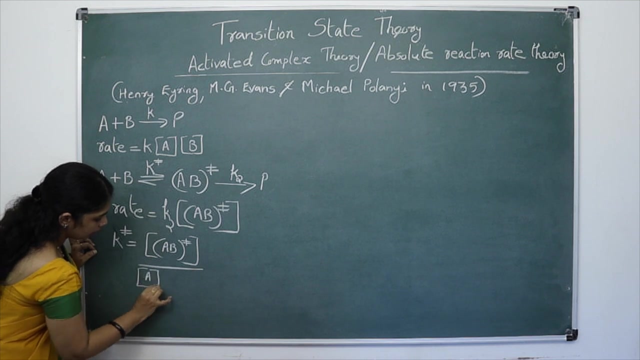 in terms of the reactants. That is, from this equation we know that the equilibrium constant is equal to concentration of activated complex divided by concentration of the reactants. Or by rearranging what will be the concentration of activated complex, The concentration of? 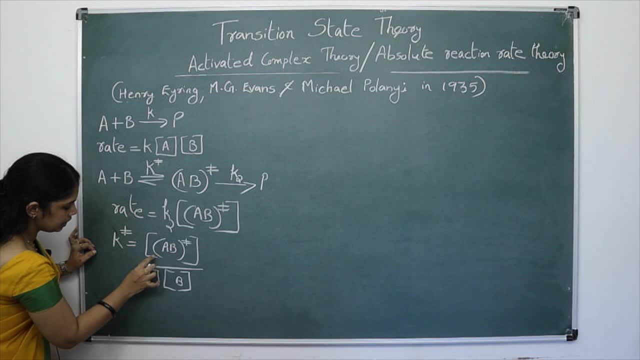 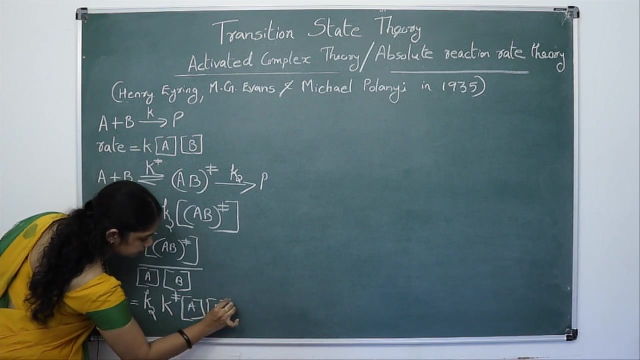 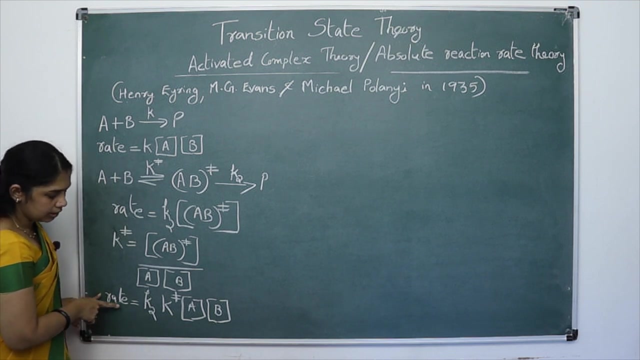 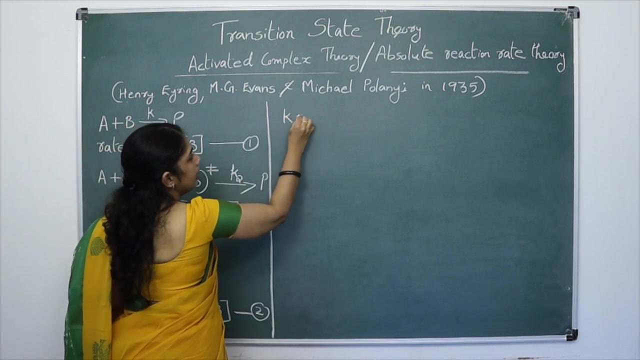 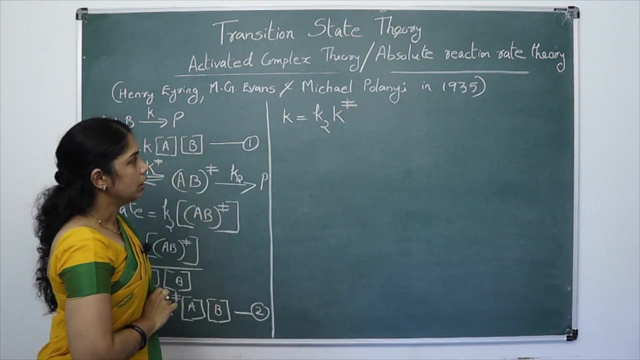 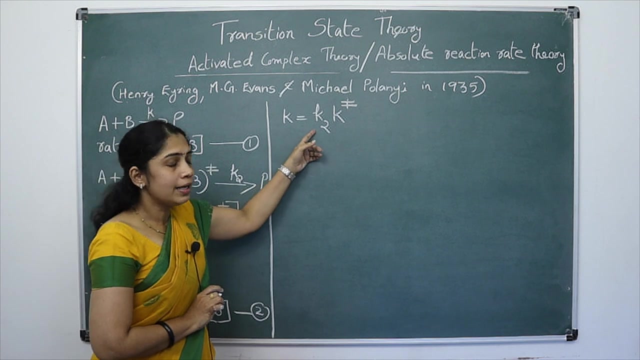 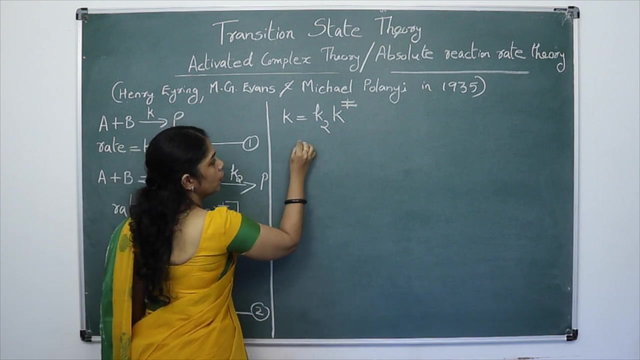 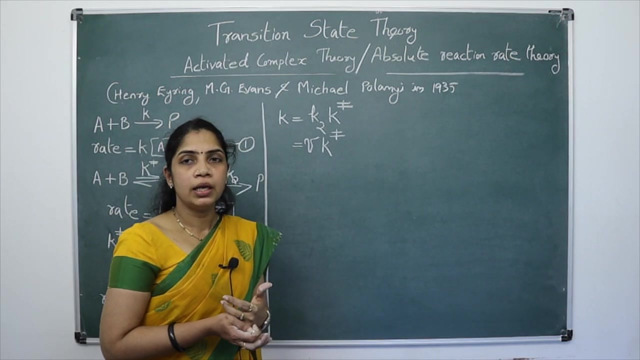 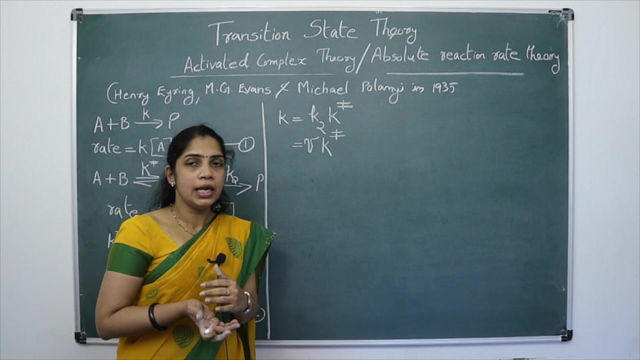 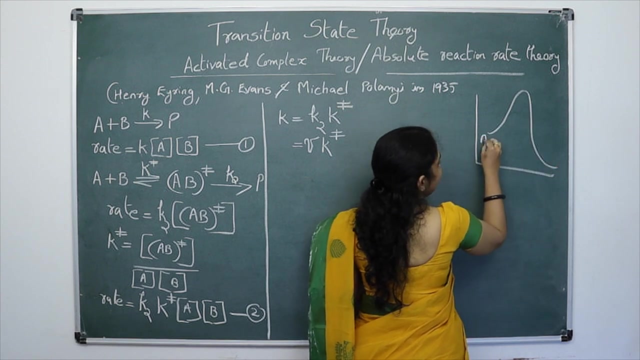 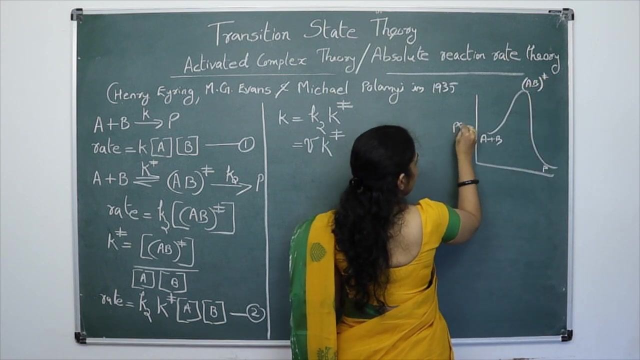 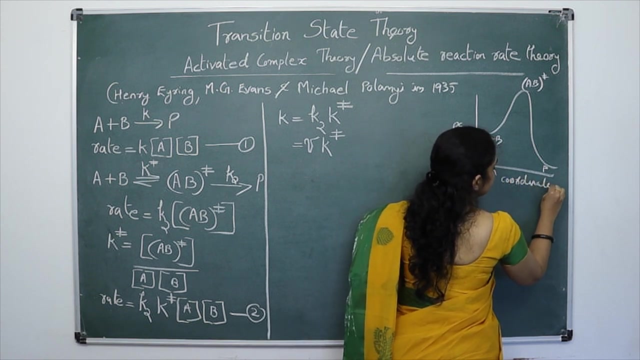 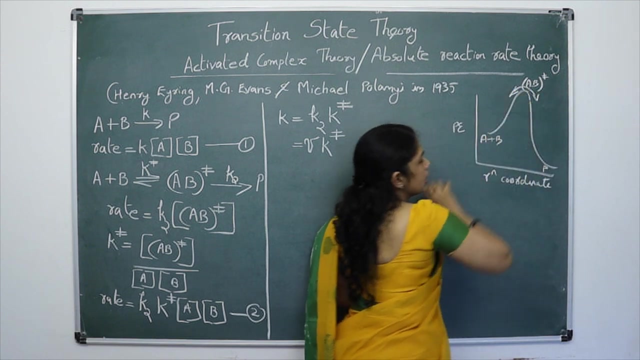 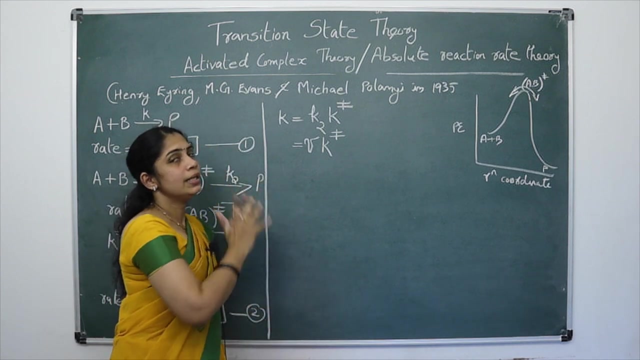 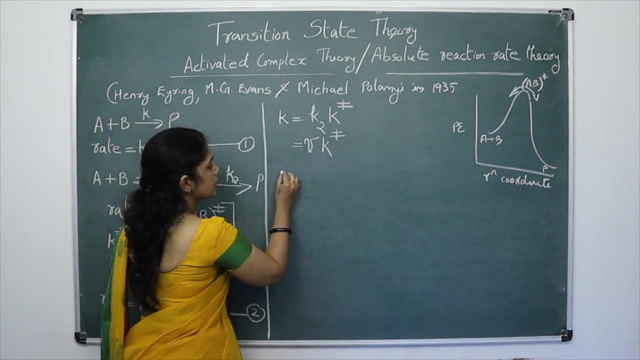 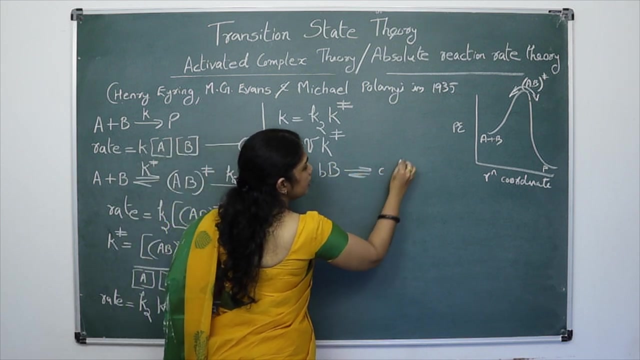 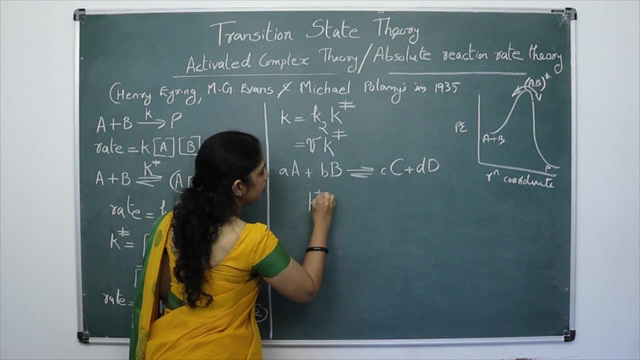 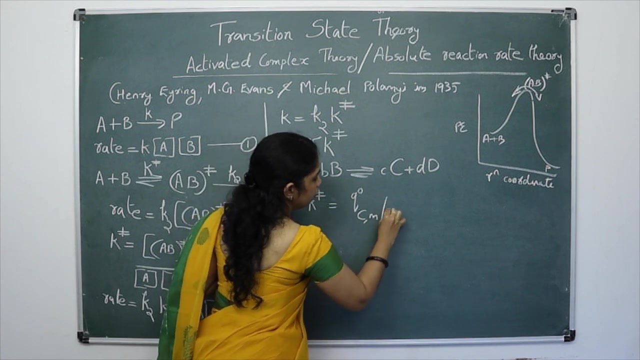 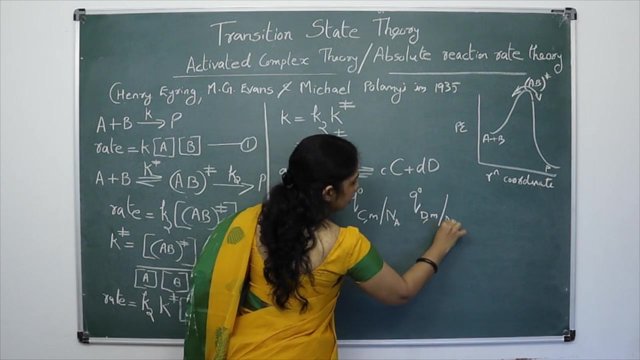 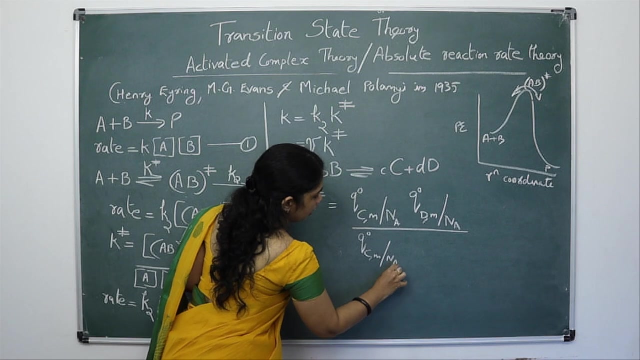 the reactants And the equilibrium constant k double dagger is equal to standard molar partition function of C into standard molar partition function of D, divided by standard molar partition function of A into standard molar partition function of D. So this is the equation, So we can. 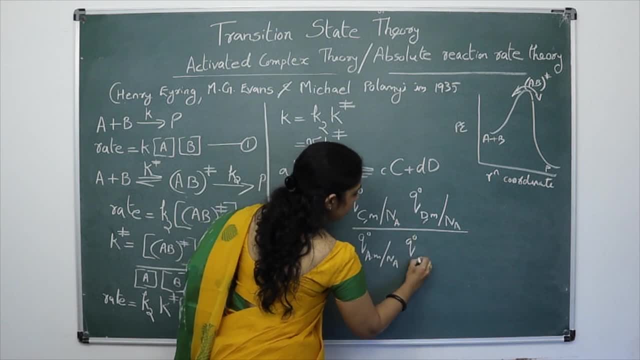 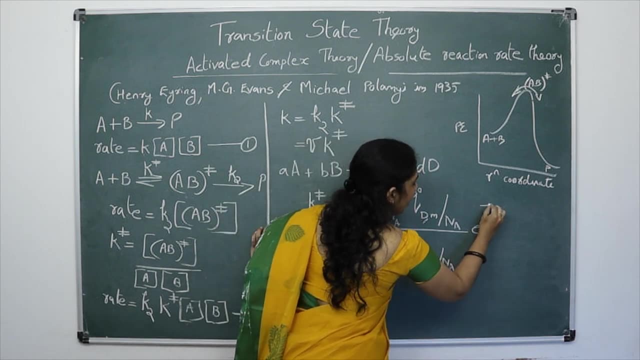 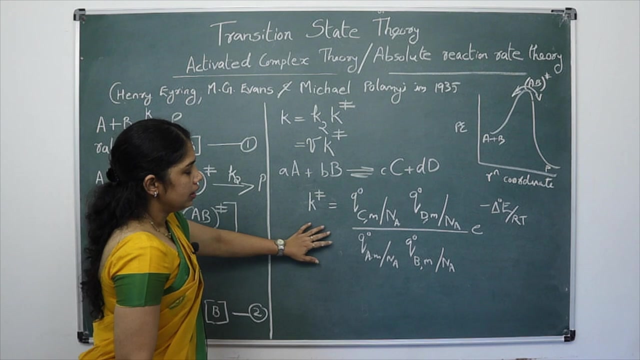 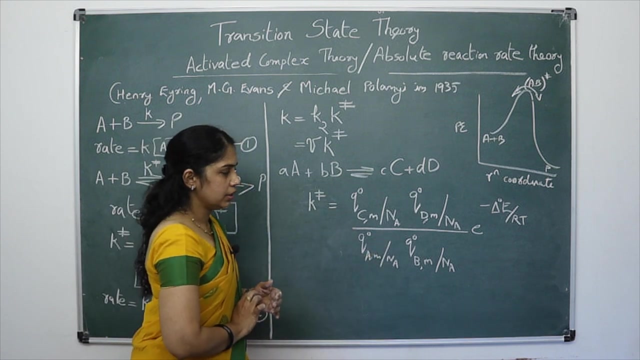 write the equation For del E 0 byipping into standard molar partition function of b into E raised to minus delta E 0 by RT. this is the general equation connecting the equilibrium constant with partition function. If you know the different states, different properties of a molecule, we can 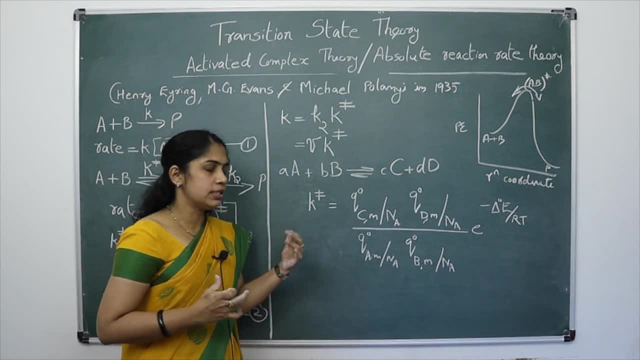 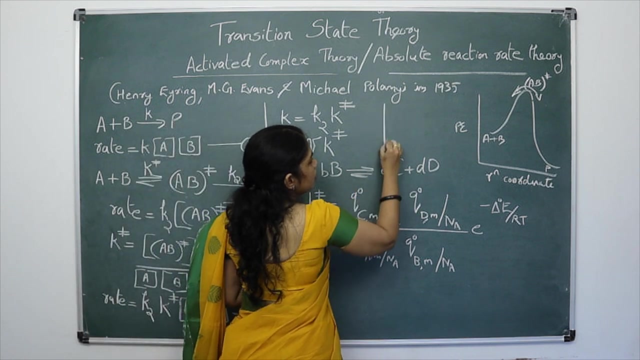 calculate of a molecule. we can predict, we can find its partition function. It gives the actual information of the molecule. Here delta E 0 is a zero point energy. What is zero point energy? Suppose these are the energy levels of the reactants and these are the energy levels of the product. 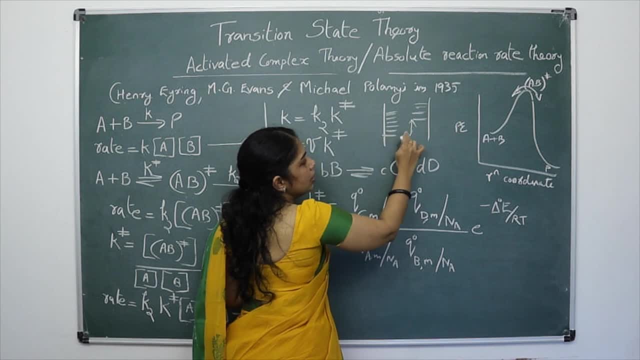 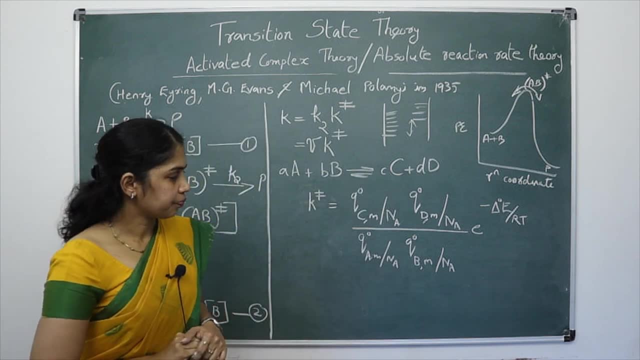 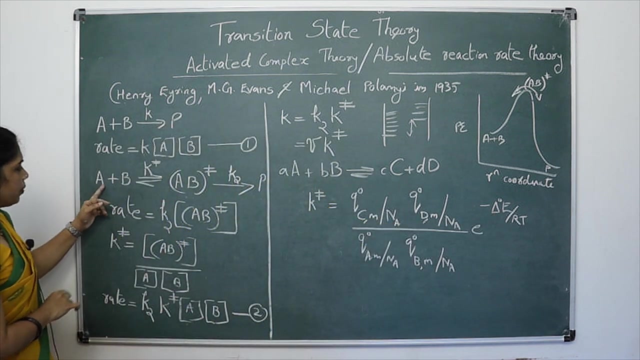 and from ground vibration energy level of the reactant to the ground vibration energy level of the product. this difference in energy is called zero point energy. So here this delta E- 0 is a zero point energy For this expression. that is A plus B in equilibrium. 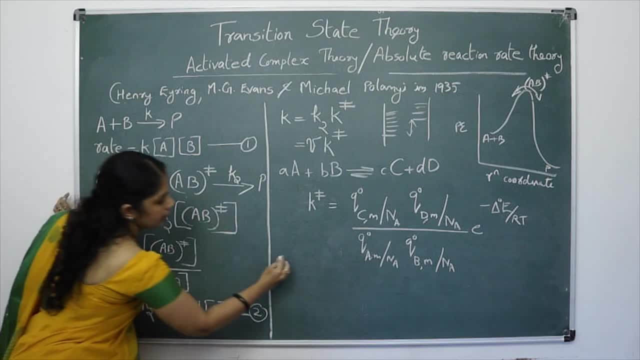 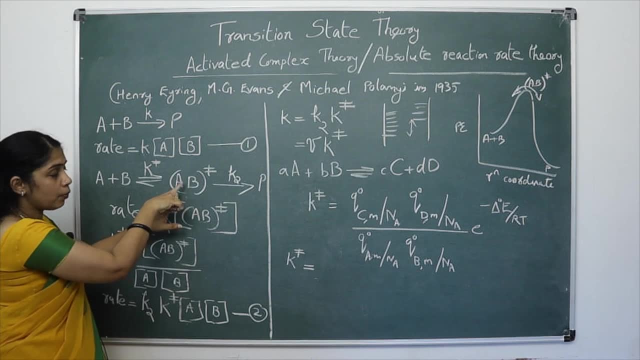 with AB double dagger. the equilibrium constant equilibrium constant K double dagger is equal to standard molar partition function of this activated complex divided by standard molar partition function of this activated complex And the equilibrium constant. equilibrium constant is multiply by delta E 0.. Here, delta E 0 is: 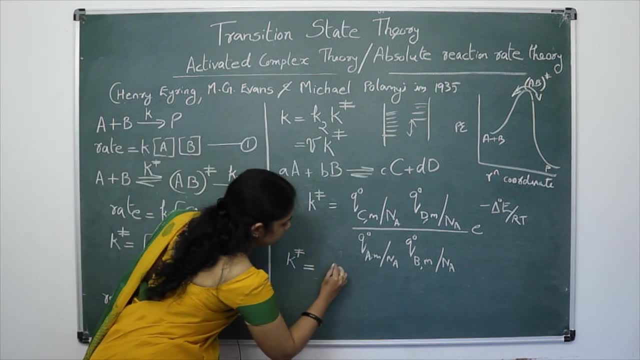 equal to delta e 0 byös delta minus delta e 0 byés delta e0 by rt. So that is the equilibrium constant. equilibrium constant, and here we have a normal equation. Here CO is meteorological equation and you can write it here the table can be 네: 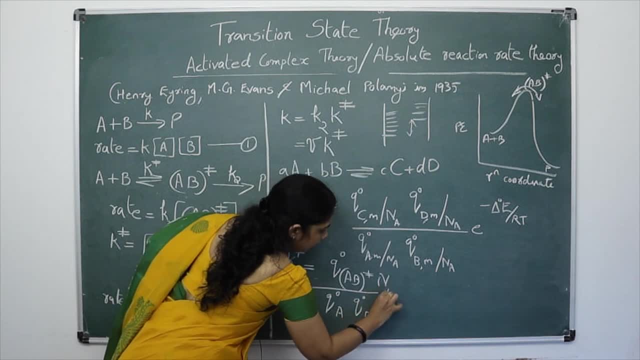 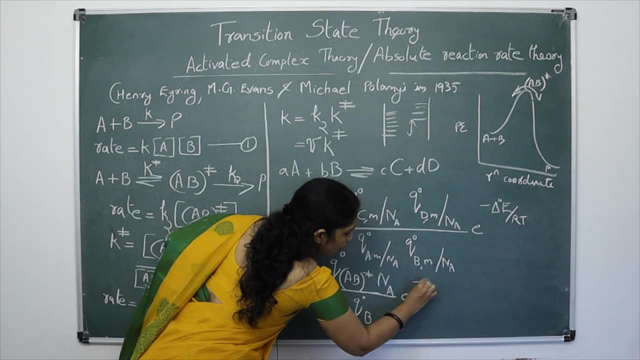 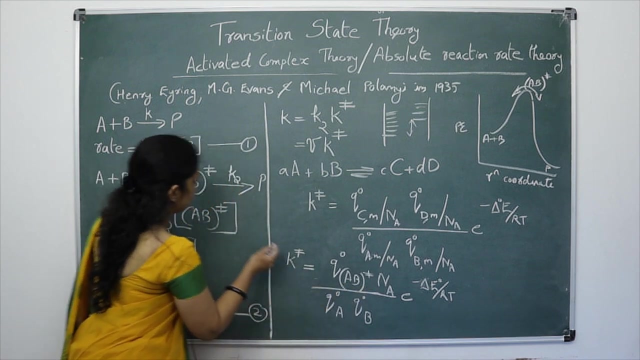 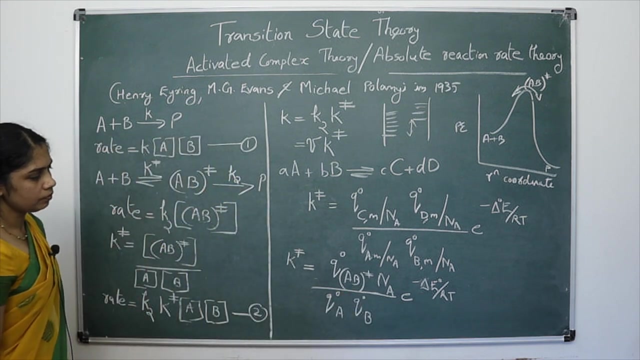 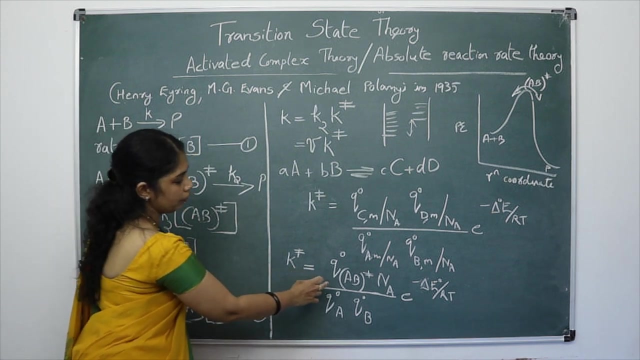 Futurable equation of limit to optimal voltage E 0, Here 1 Na, because here 2 reactants and 1 product, so Na Na getting cancelled and 1 Na remains here. So we got the expression for equilibrium constant in terms of partition function. 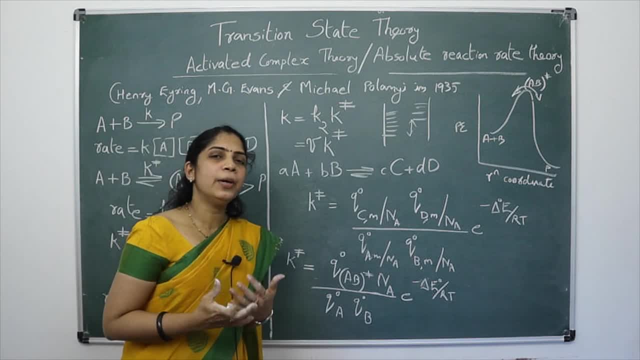 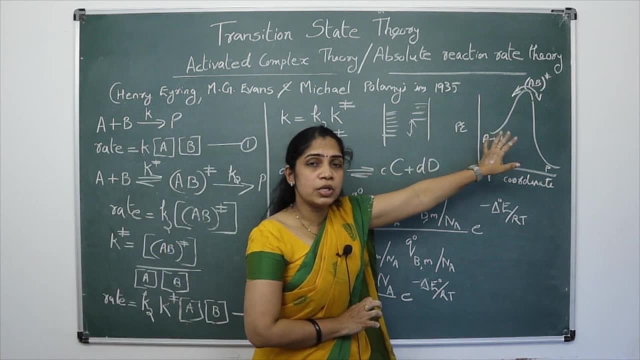 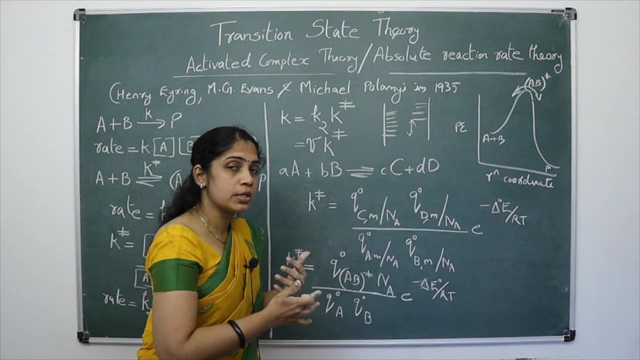 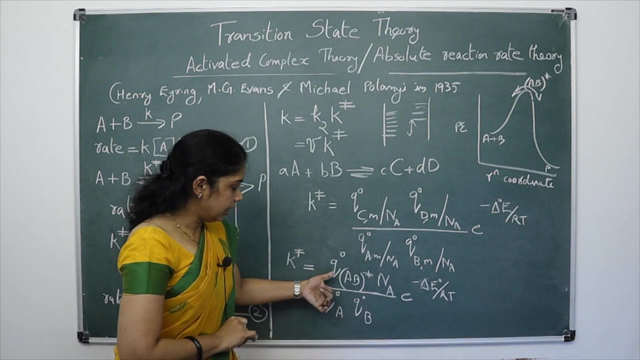 The third conceptual lead made by Polanyi is that actuated complex formation. actuated complex formation. the reason for the actuated complex. actuated complex formation is is their asymmetric mode of vibration, That is here in this term, that is partition function of this actuated complex formation. 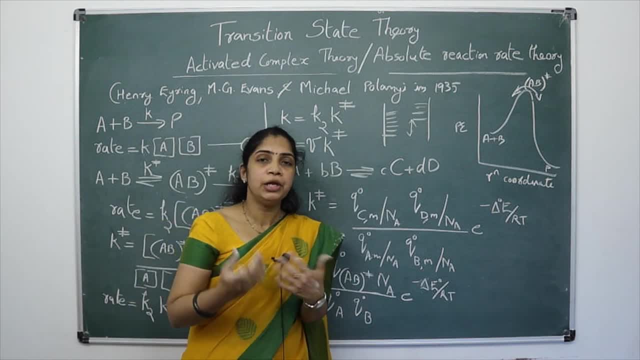 of this actuated complex and this partition functions can be different types, that is rotational partition function, translational partition function, then vibrational partition function, etcetera. So this is the product of old old, that is rotational, translational, vibrational, etcetera. 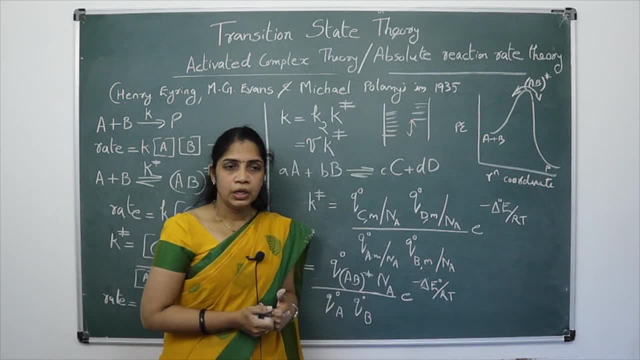 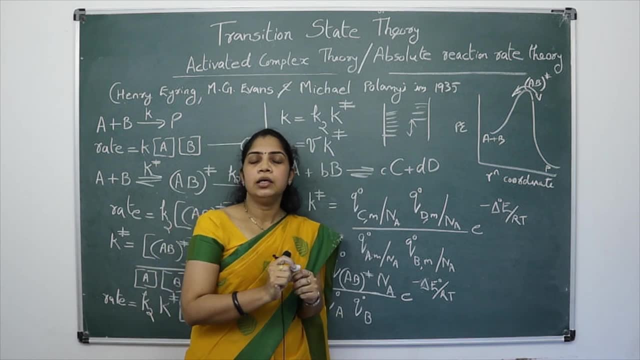 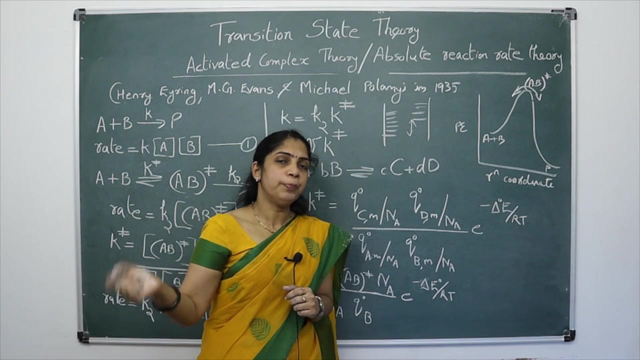 This is the product of old types of degrees of freedom, but the conceptual lead they made is that the one particular function of this actuated complex formation is called vibrational partition. One particular degree of freedom, one particular vibration, is a reason for the formation of 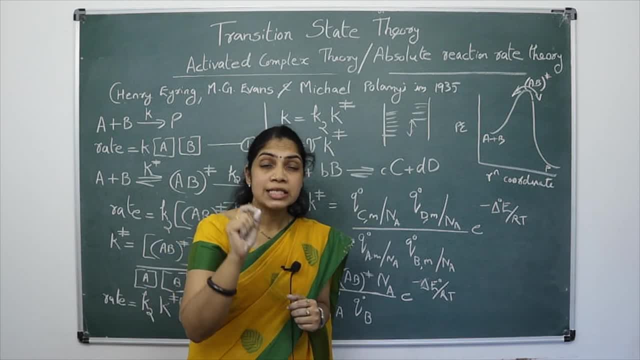 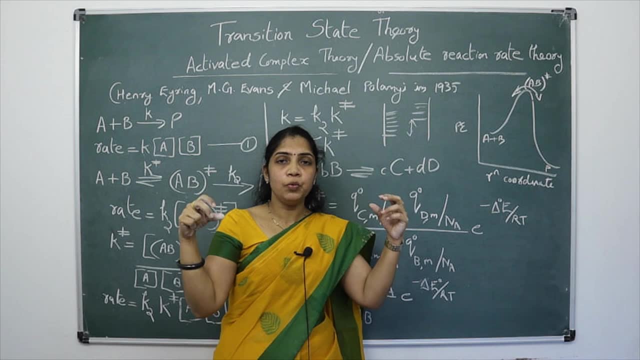 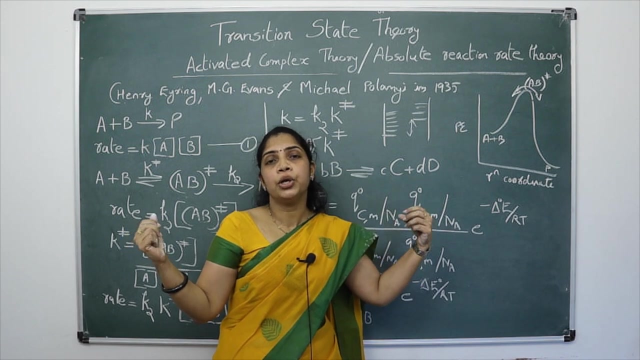 the product. that is asymmetric mode of vibration. that is actuated complex. In the case of actuated complex, the actuated complex is a species in which there is reactant and product and here the reactants. reactant bond is going getting consumed and product. 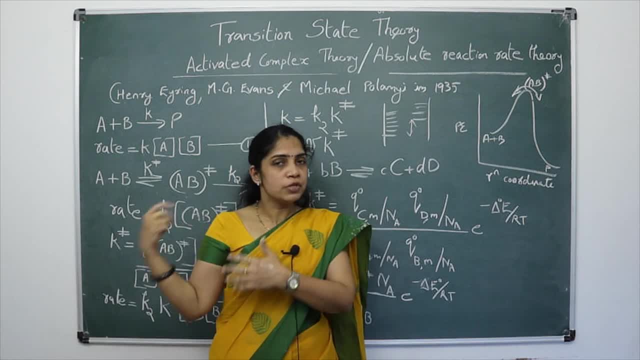 bond is produced. So this is the product of the product. Product bond is formed and the reactant bond is getting consumed. So it is a type of asymmetric mode of vibration that that happens, or that that is a critical point, or that is a reason for the formation of the product. 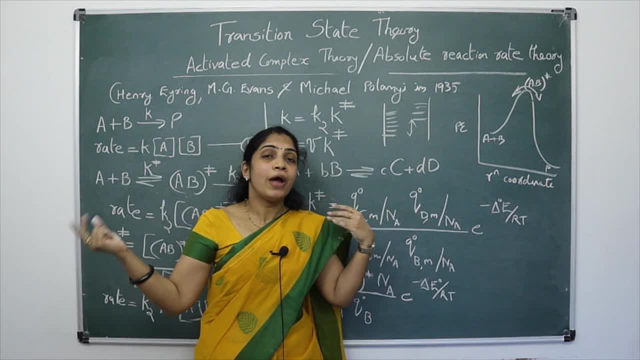 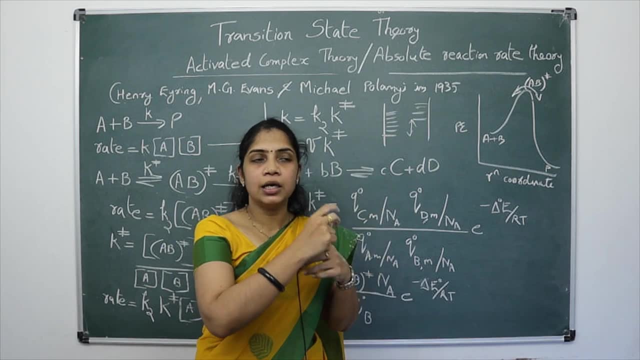 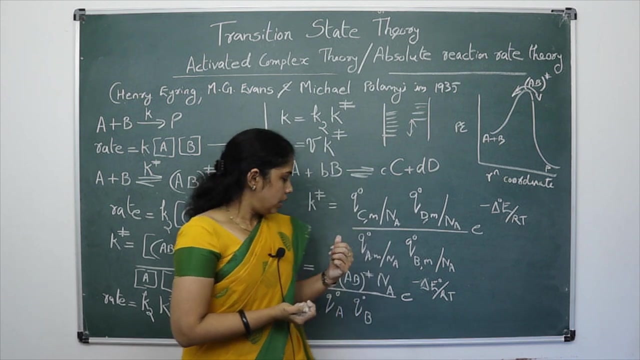 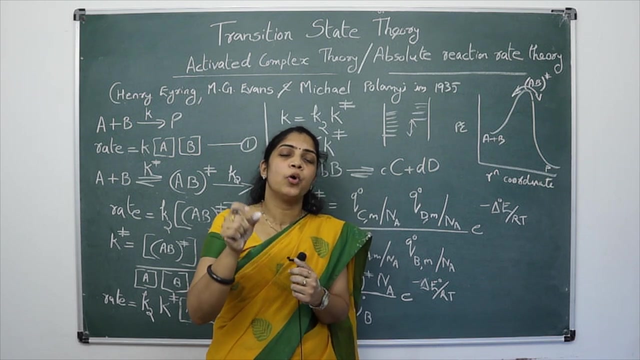 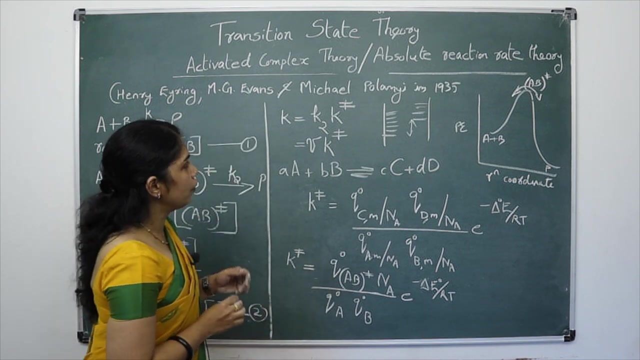 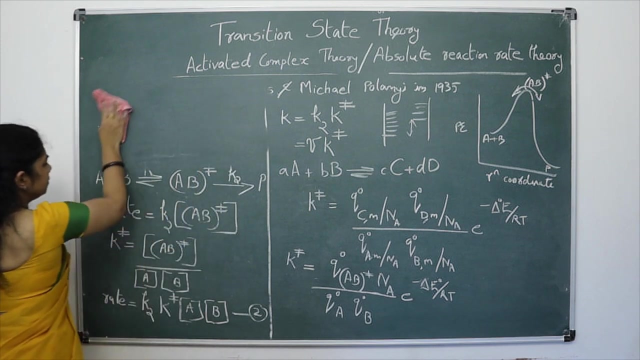 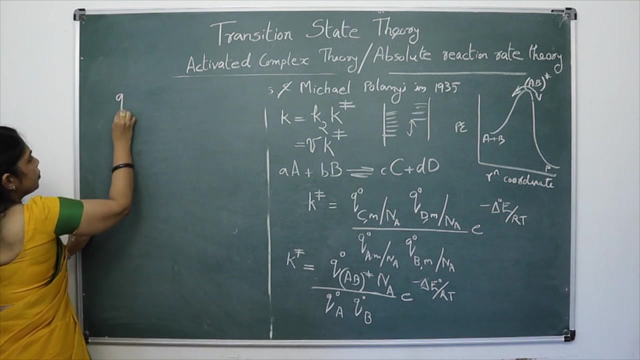 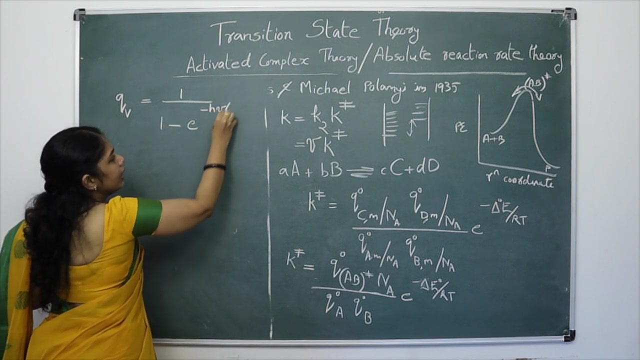 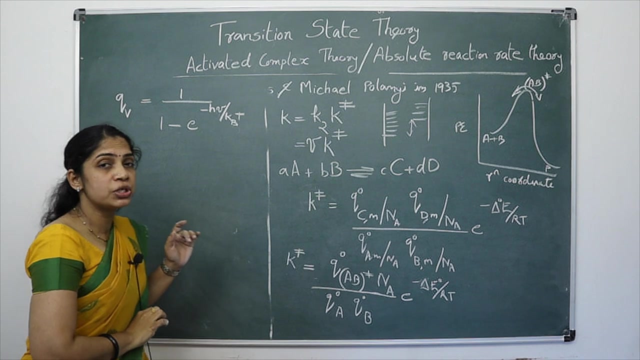 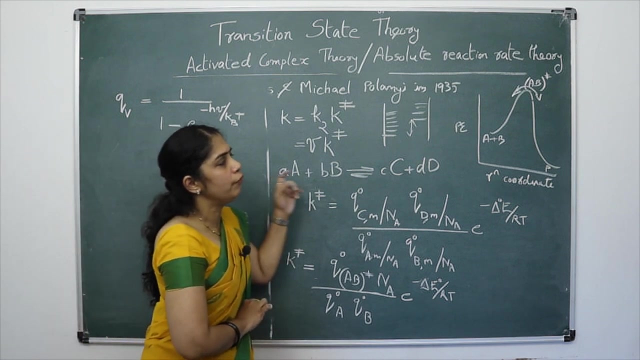 So they made a special contribution, special contribution made by the asymmetric mode of vibration. And here the number of reactantsyn тр, That is, here, k is a Boltzmann constant. This is the expression for vibrational partition function. And what about the vibrational frequency of this actuated complex? Is it a that is? 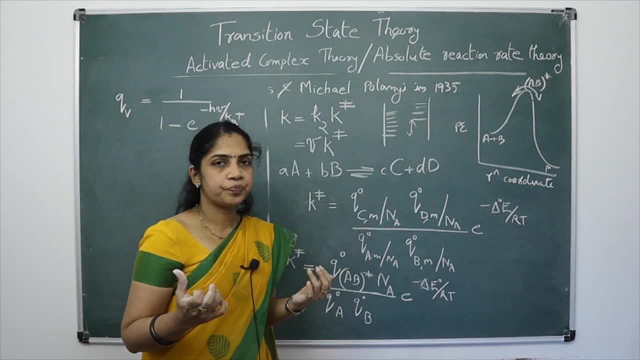 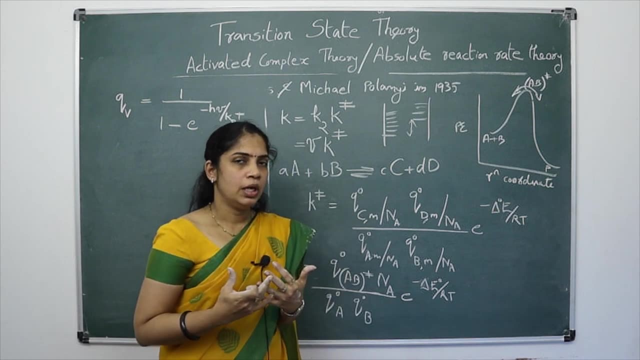 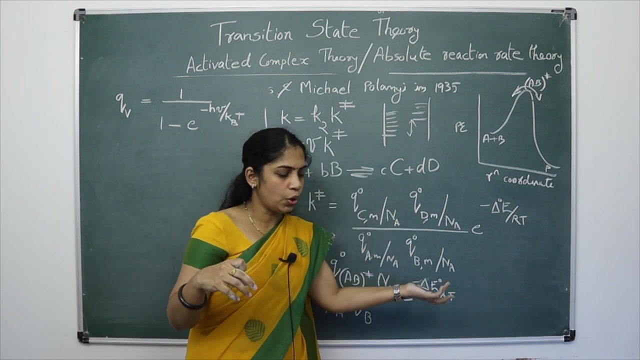 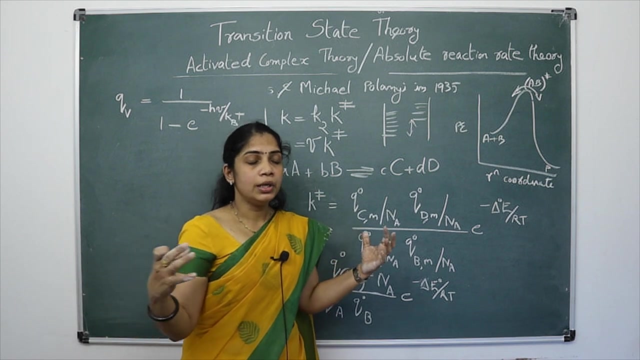 it a weak frequency or it is a strong frequency. It will be a weak, weak mode of vibration because here, as I already discussed, as I already told, that is, bones are get going to decompose and new bones are going to formed. In such a situation, their frequency of vibration is 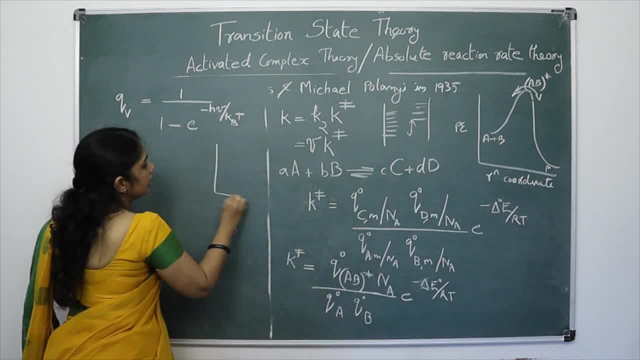 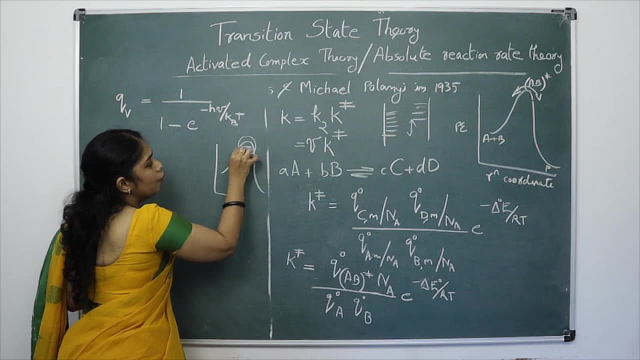 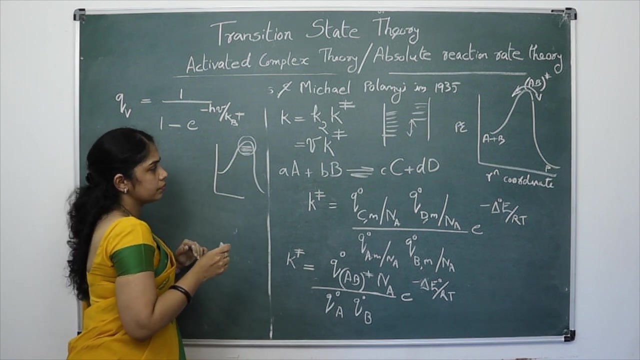 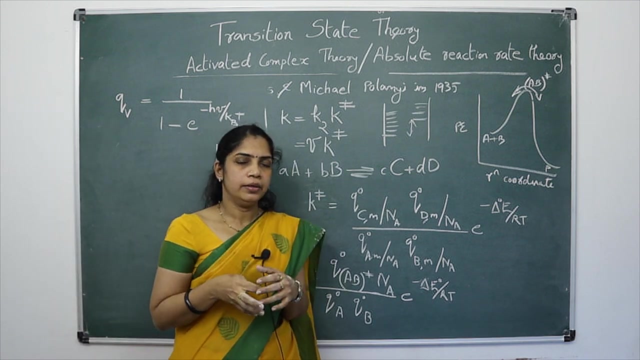 very weak and or we can say that their potential energy. in the potential energy diagram, the energy levels are are very close together and their frequency of vibration is very small. This actuator complex is situating in the, this potentiometer energy well and energy. 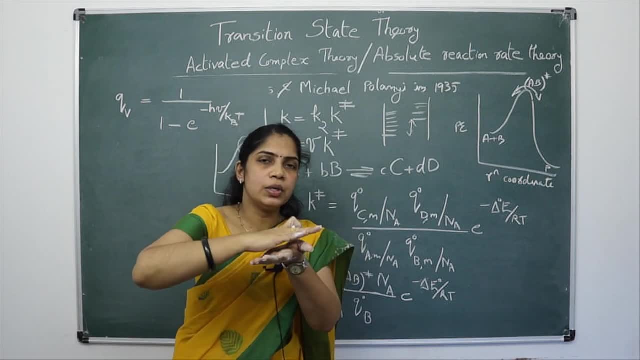 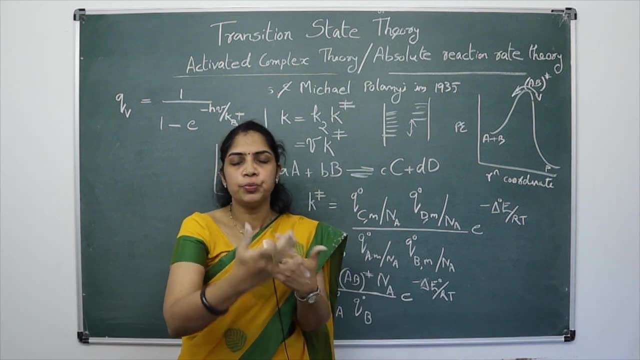 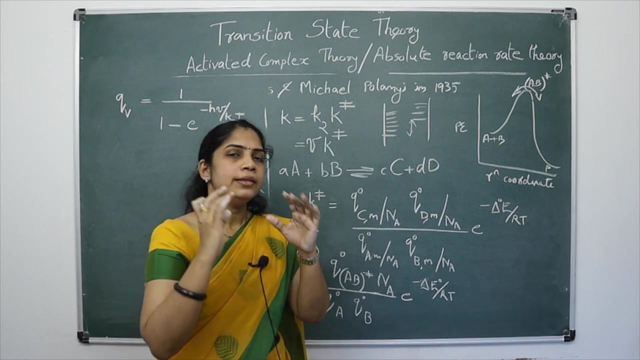 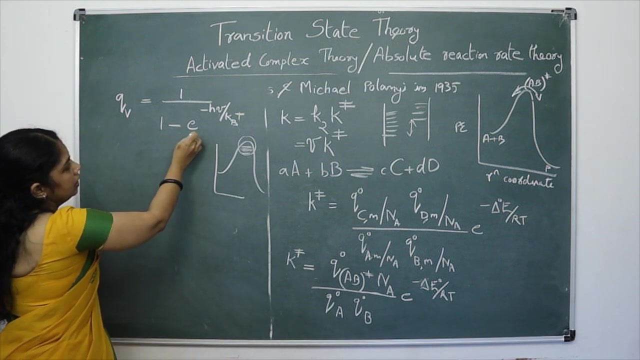 levels are closely packed and their frequency is very low and we can say that it is a soft mode of soft type or soft mode of vibration or super soft mode of vibration. So that that takes that, takes into expand this e raise to minus x term. 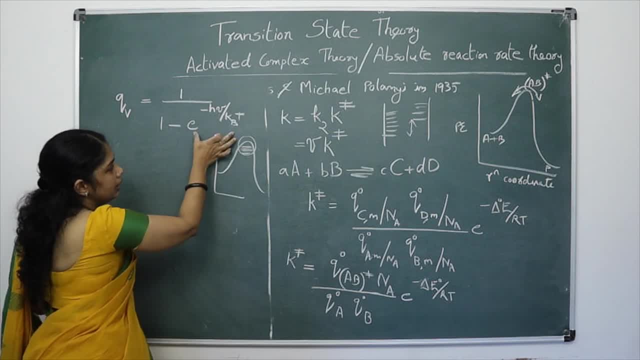 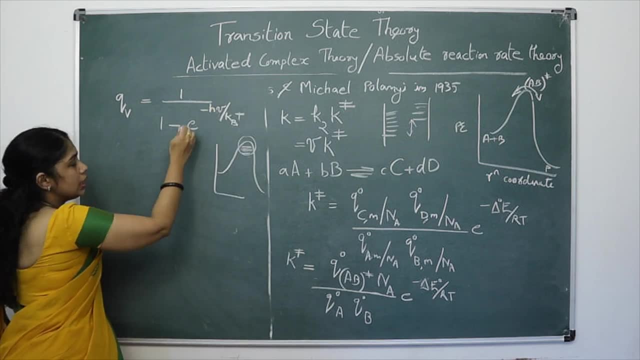 This is an e raise to minus x or e raise to minus h, nu by k, B, T. This make us to expand this term. What is a expand Expansion of? e raise to minus x, e minus minus? e raise to minus x is 1 minus x plus x square. 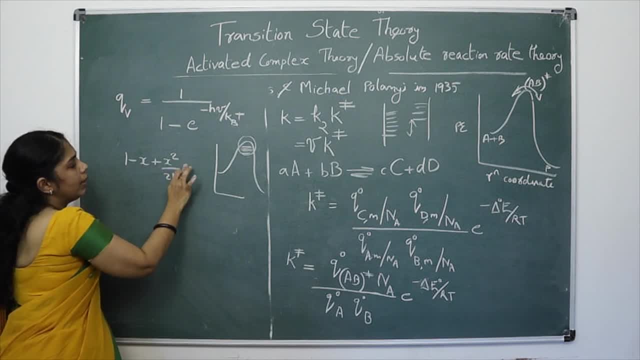 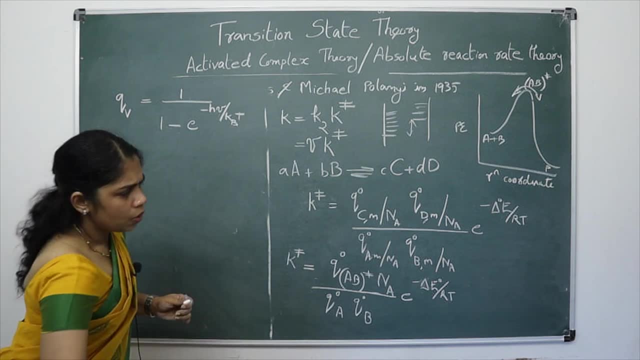 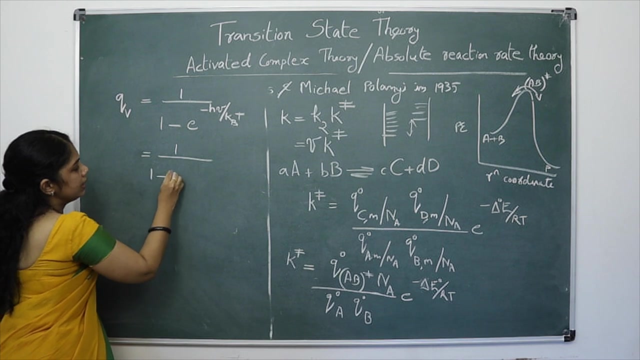 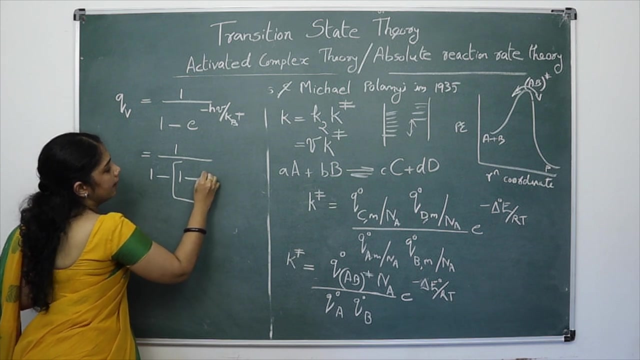 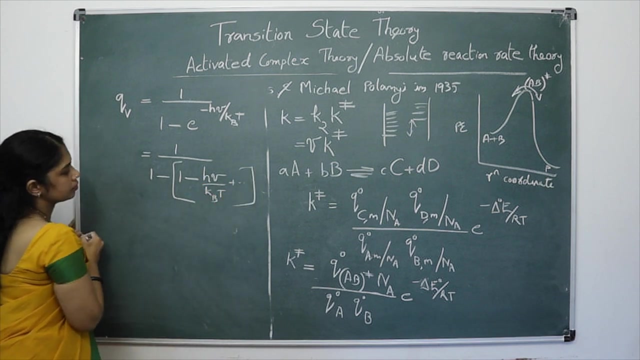 by 2 factorial minus etcetera. So on expansion of this series, we get 1 divided by 1 minus e raise to x. expansion of e raise to minus x is 1 minus 1 divided by 2 factorial. So we get 1 minus 1 minus h, nu by k, B, T plus etcetera. 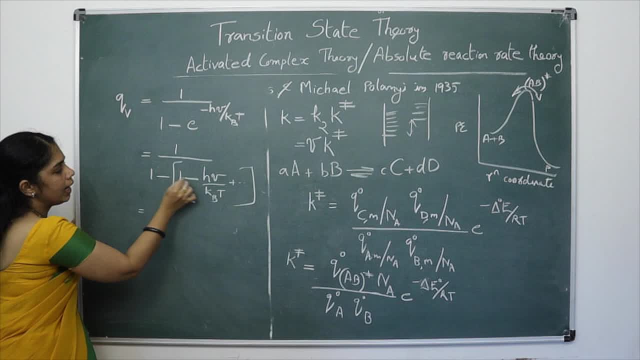 On rearranging this 1, 1, 1 minus 1, 0 and this is plus, and on rearranges we get k B T by h nu as a expression for vibrational partition function 1 minus 1 minus h nu by k B T by h nu. 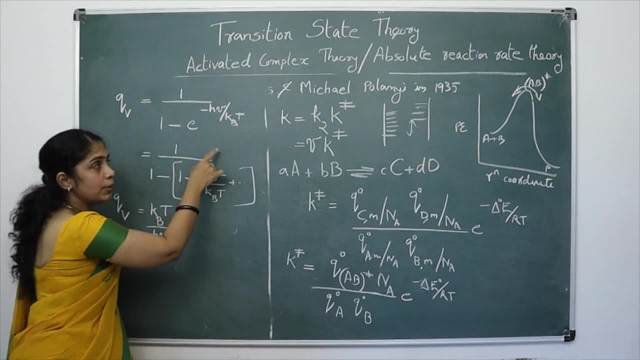 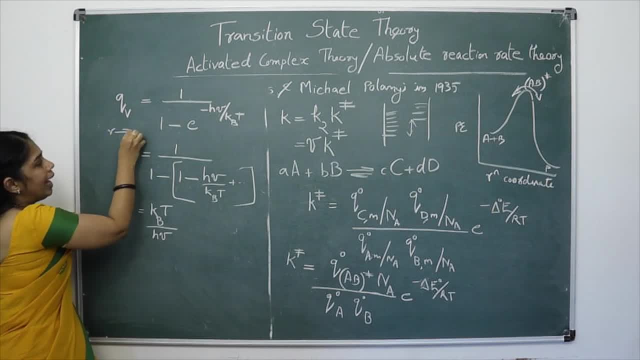 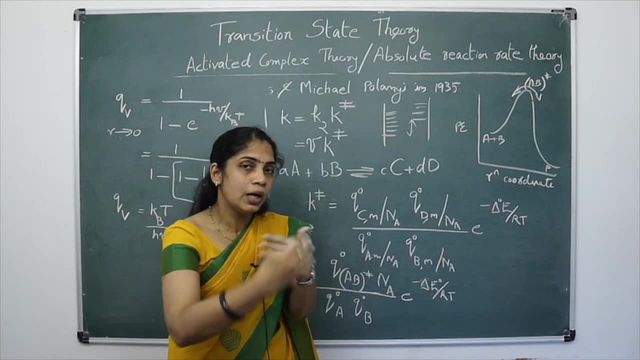 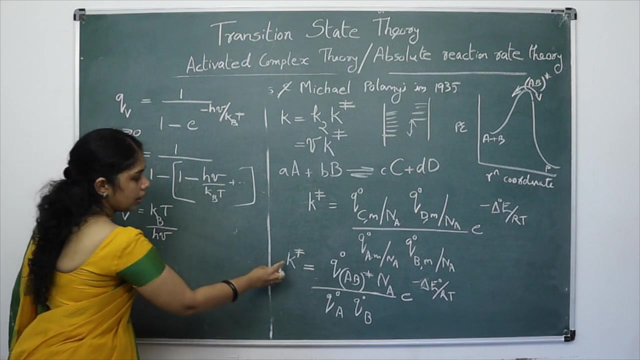 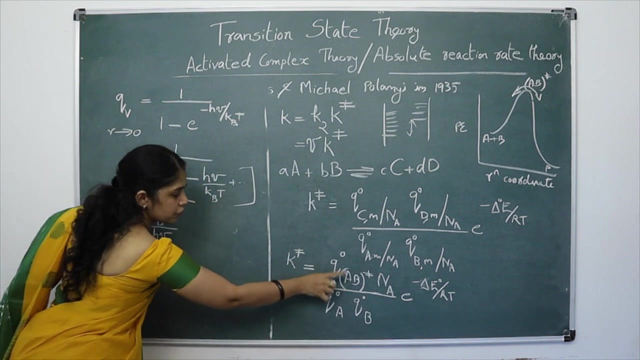 Because here the frequency nu approaches to 0. It is a weak mode of vibration that frequency approaches to 0. that allows us to expand this series and we get the value as k, B, T by h, nu. Now we can write the value of this partition function, that is, partition function of actuator. 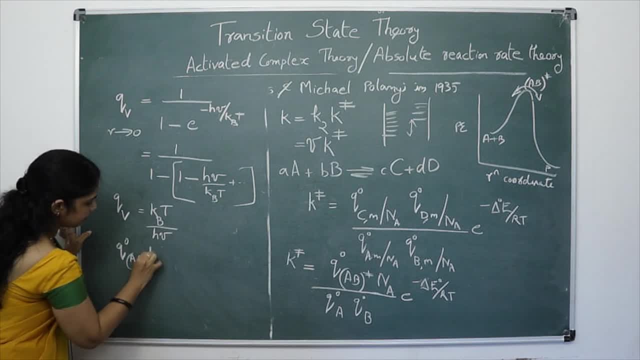 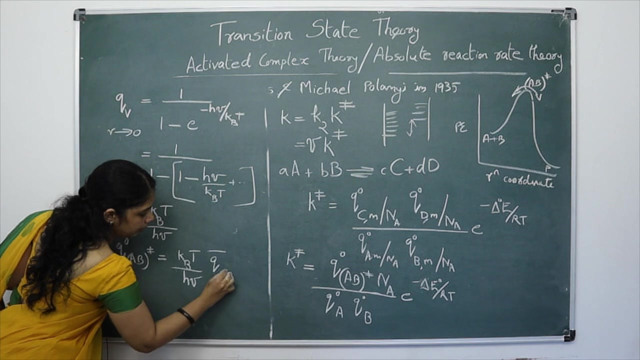 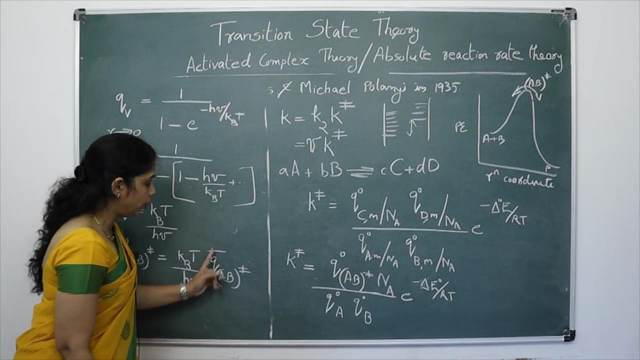 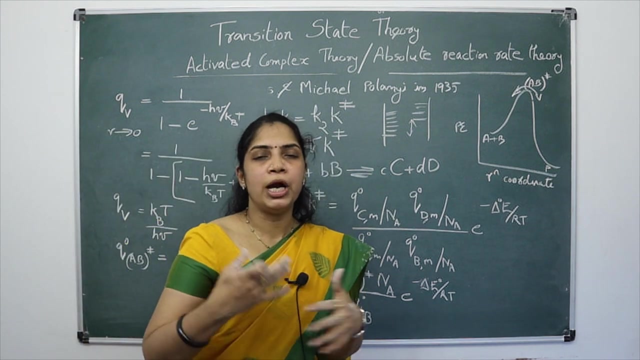 complex. partition function of this actuated complex is equal to kB T by h nu into q bar a b double dagger. What is this nu term? that is, q bar a, b double dagger. I already said there are different types of partition functions or there are different types of degree of degrees. 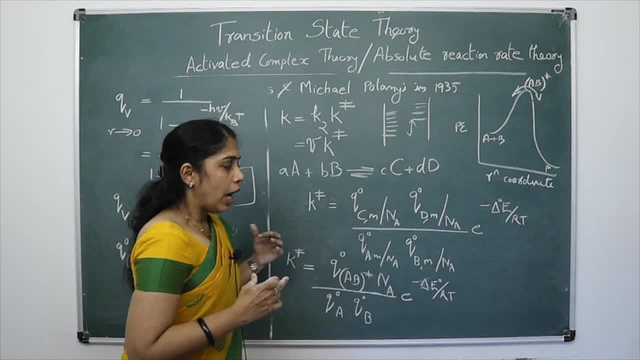 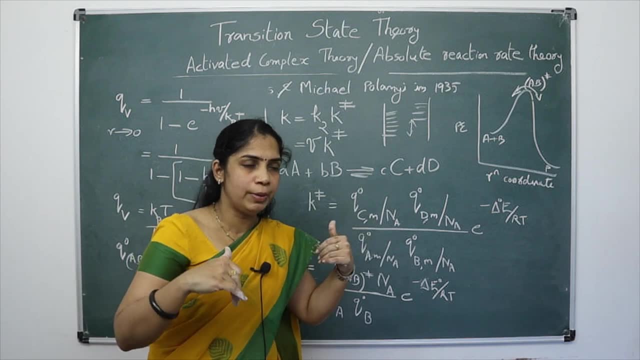 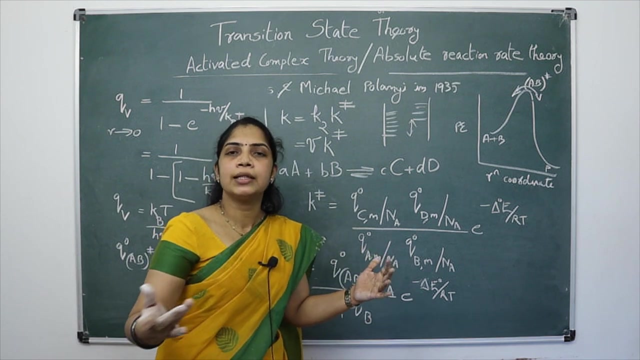 of freedom, that is rotational, translational, etc. And we here excluded one term, that is asymmetric mode of vibration. asymmetric mode of vibration, All other vibrations, that is symmetric vibration. And other degrees of freedom, that is rotational, translational motion, rotational motion, etc. 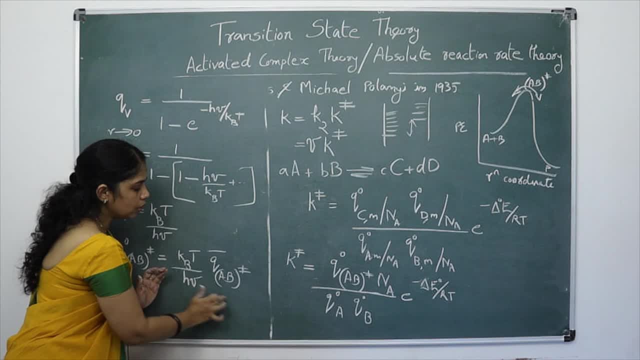 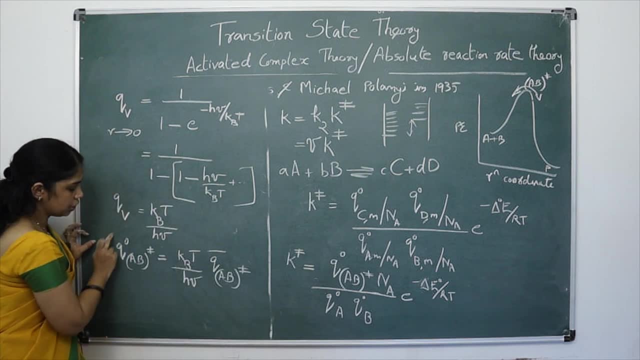 is there. So this term includes all other terms excluding the asymmetric mode of vibration. So the partition function, total partition function of the actuated complex is the partition functions, partition function due to the asymmetric mode of vibration and all other degrees of vibration. 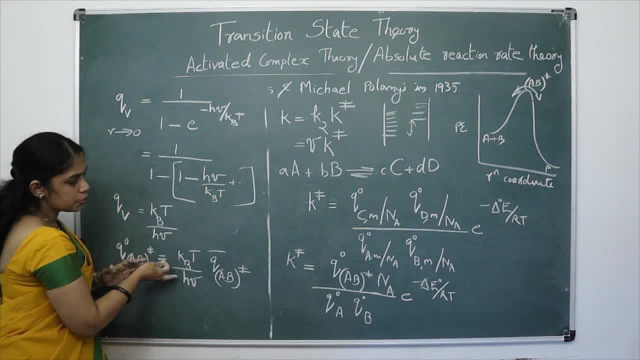 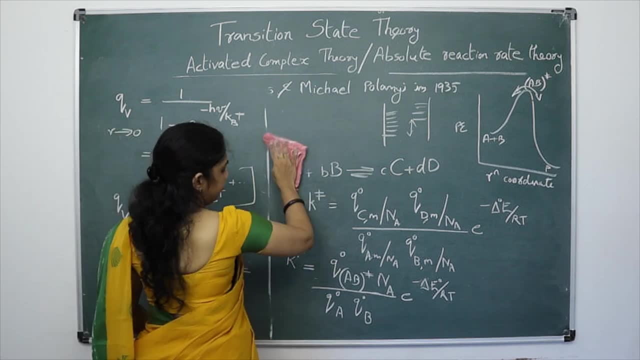 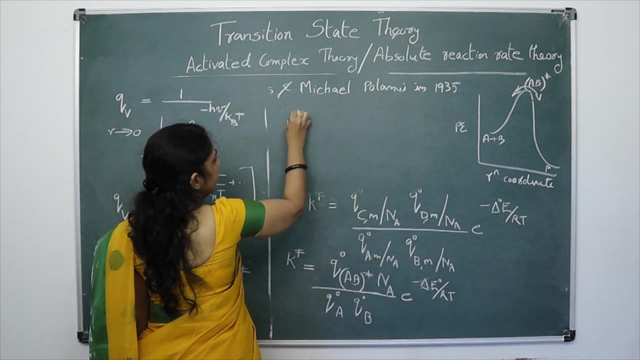 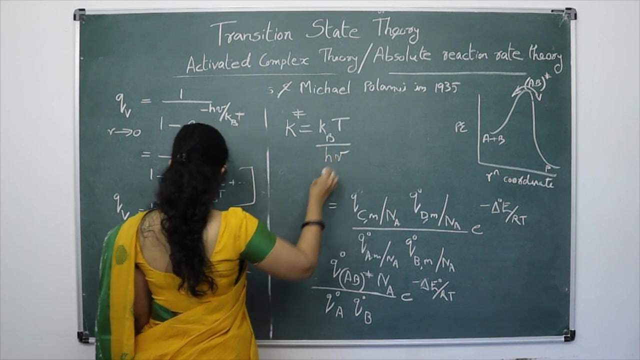 And this partition function is the partition function of all other partition functions. On substituting this value into this equation, that is the equation of equilibrium constant k double dagger is equal to kB. T by h nu into q bar of actuated complex, the equilibrium. 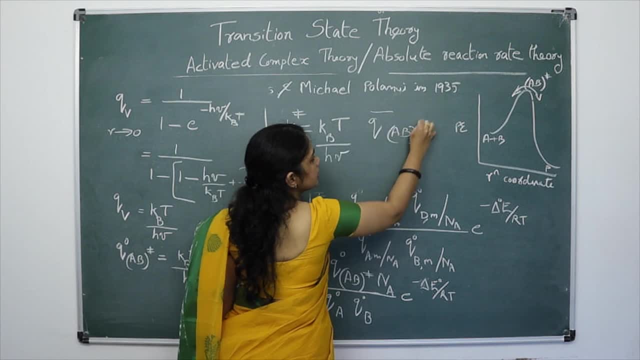 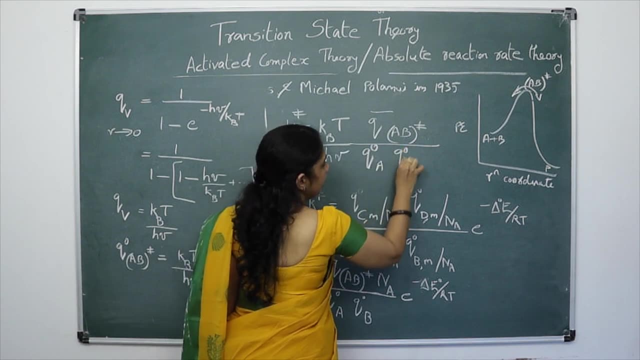 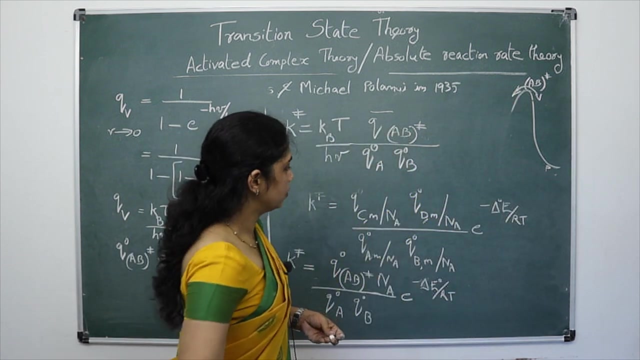 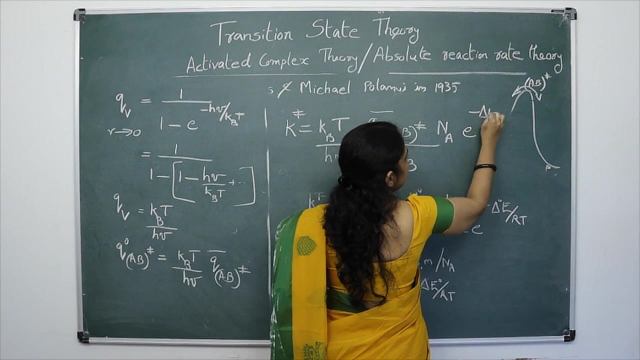 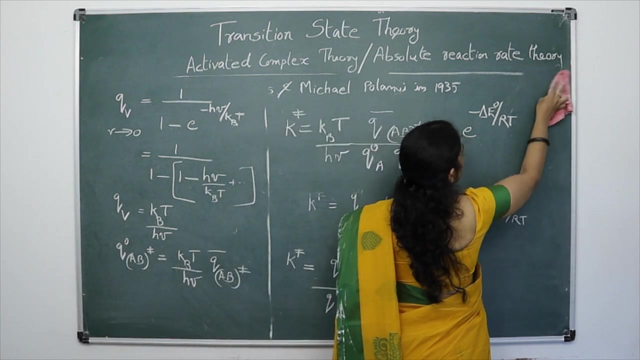 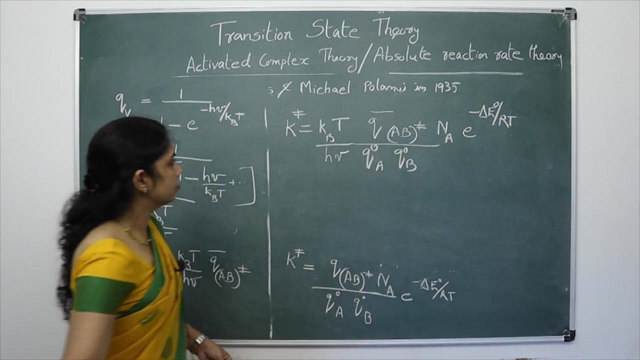 function. So the equation is this: Thank you. x divided by Q0 of A, into Q0 of B, into NA, into E, raise to minus delta E0 by Rp. okay, This is the expression for equilibrium constant and we, if we replace this, Boltzmann constant, 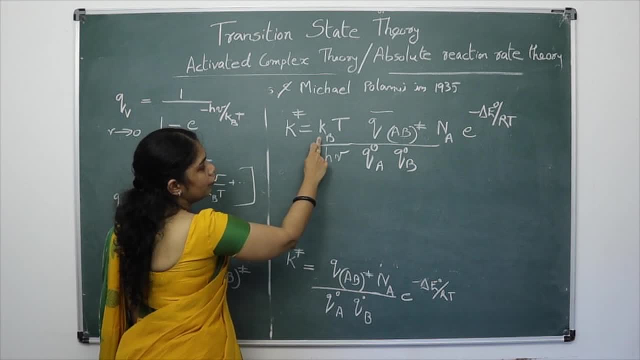 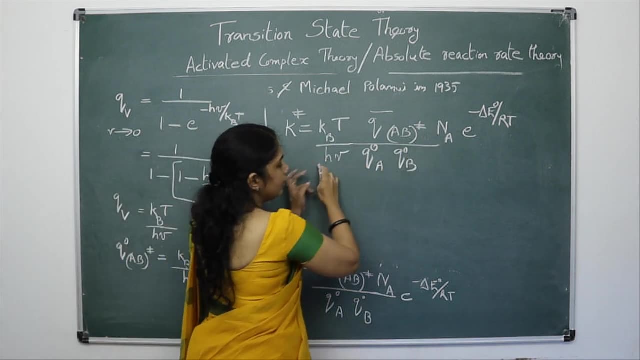 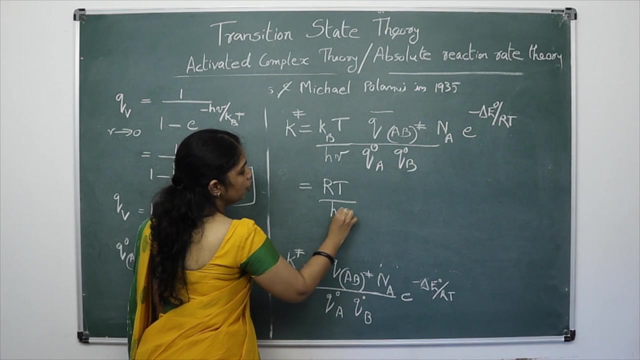 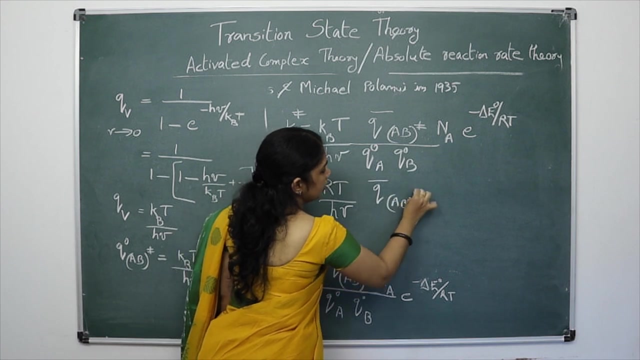 with universal gas, constant R, we can write it as R by NA. then here, this R by NA and this NA and the denominator NA will be cancelled, and this will be cancelled, Okay, Okay, And the expression become Rt by h nu into Q, bar, AB, divided by Q0 of A, into Q0 of B, into 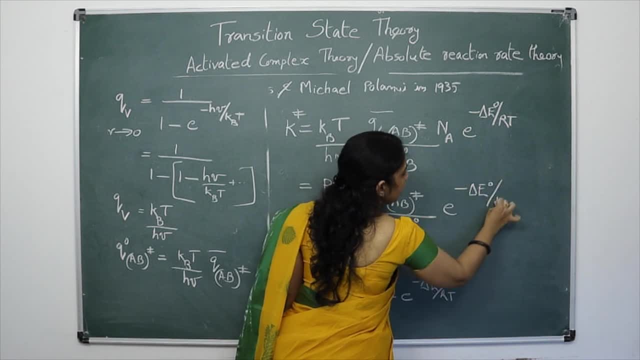 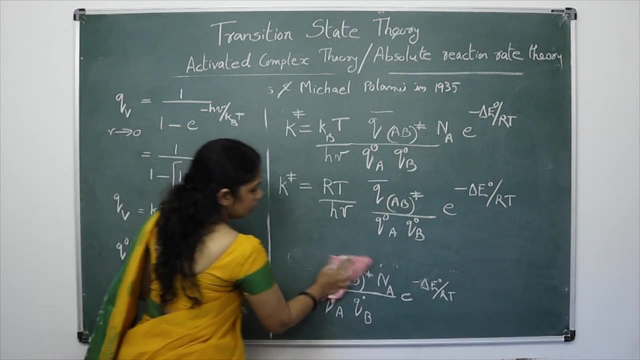 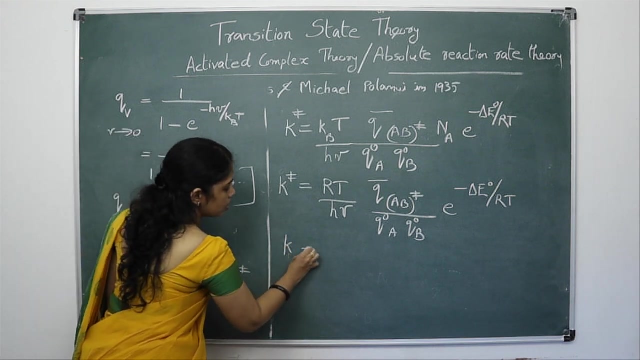 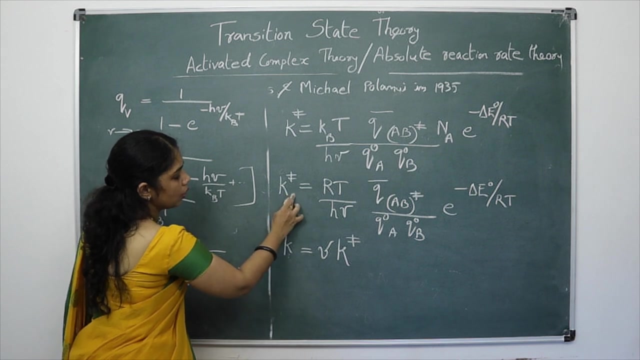 E raise to minus delta E0 by Rt. This is the expression for equilibrium constant. Then what is the expression for the general? The general rate constant that we find at the beginning, that is, rate constant, is equal to nu, into equilibrium constant. On substituting this equilibrium constant in the in this expression, we get this nu. 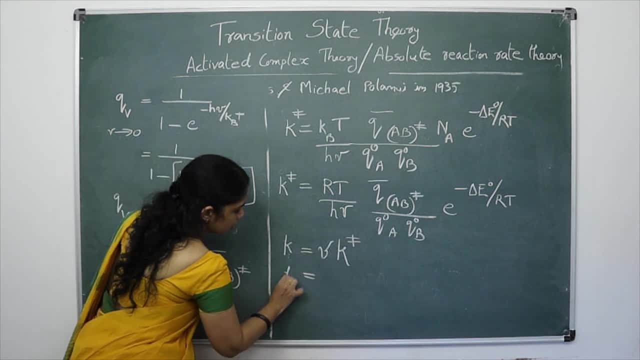 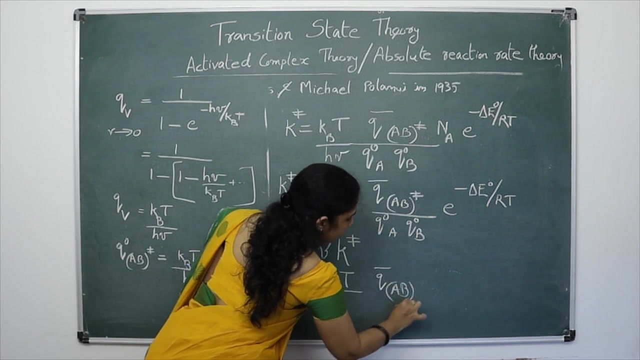 and nu get cancelled. So rate constant K is equal to Rt divided by h. So we are doing that, we are getting that. we are getting as we write it. as what is the equation? The equation is: just write this as Mu over Theta P: 0. 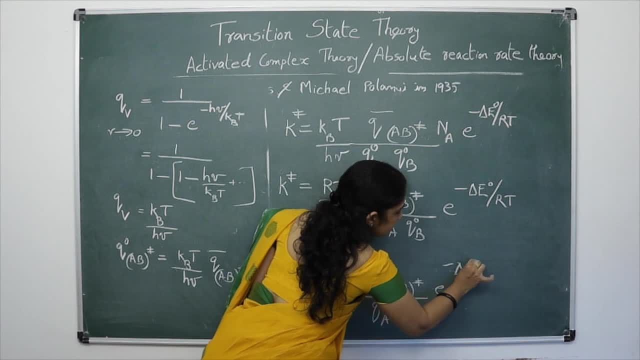 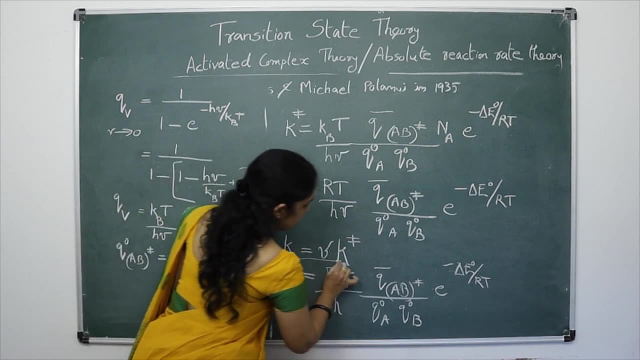 B into delta X, into two bar of activated complex divided by Q0 of A into Q0 of B, into E. raise to minus delta E0 by Rt. So this is the expression for rate constant. This is the expression for rate constant as per transition state.